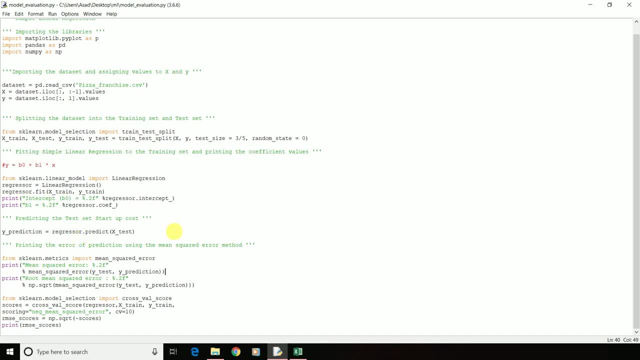 test values. Now I'll be focusing on what is actually the model evaluation path. So we used a particular function called mean squared error. What is mean squared error means? Mean squared error is a popular formula to measure the error rate of a regression model. However, it can only be compared between models. 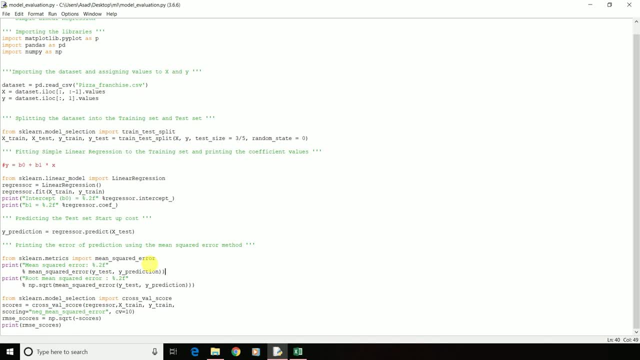 whose errors are more than the error rate of the regression model. So we have imported the mean squared error function from sklearnmetrics and we have passed our actual Y testing data and our prediction data. This will calculate the mean squared error and then I have done the square routing of it, which will give: 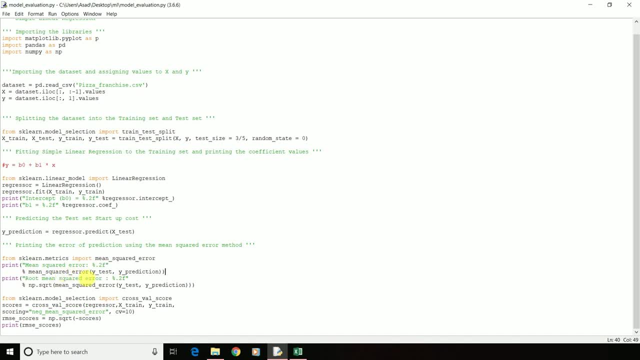 us the square root of mean squared error. The minimum this value is, the good your model is. One more great alternative for regression evaluation is scikit-learn's cross validation feature. This particular code is a k-fold cross-validation. It randomly splits the training set into 10 distinct subsets called folds, Then it trains and 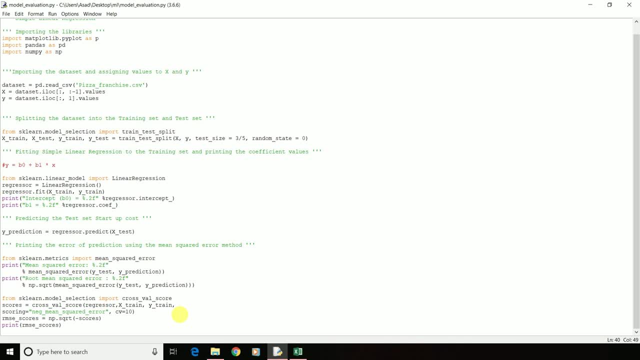 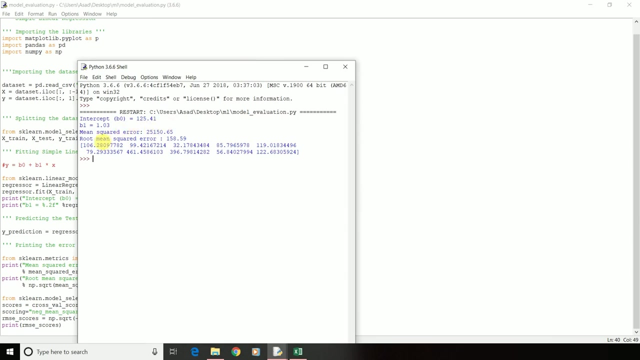 evaluates the model 10 times, picking a different fold for evaluation every time. The result is an array containing 10 evaluation scores. Now let's run this script. So I've got my mean squared error as this, and then doing the square root of the mean. 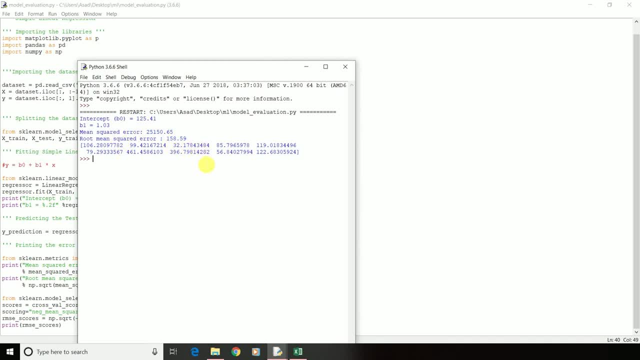 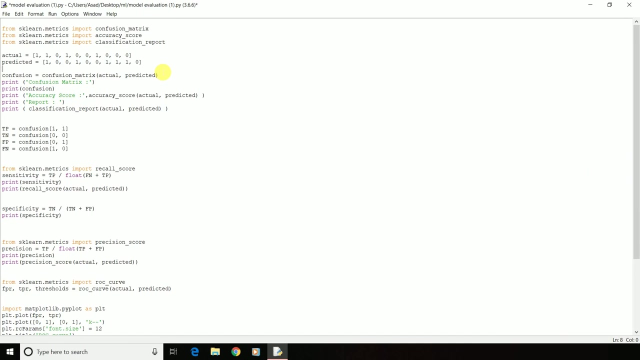 squared error, I've got 158.59.. The next output is our cross validation output. This implementation, In which each of the folds RMSE scores- that is, the root mean square scores- were calculated. Now let's move on to classification evaluation. Now consider: we have a binary classification and this is my actual values and these are my predicted values. 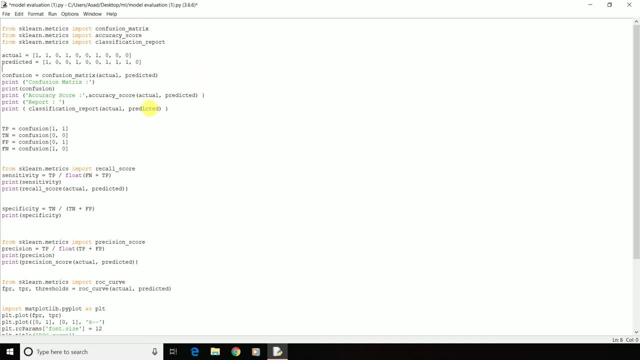 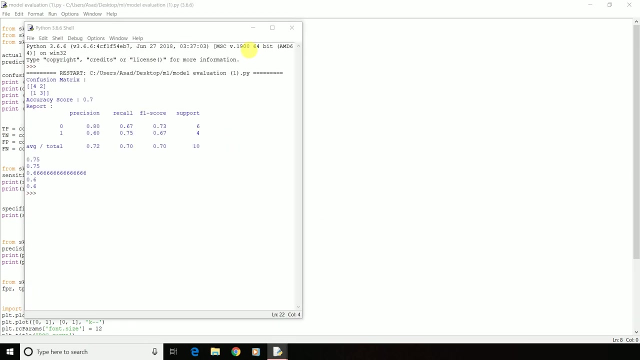 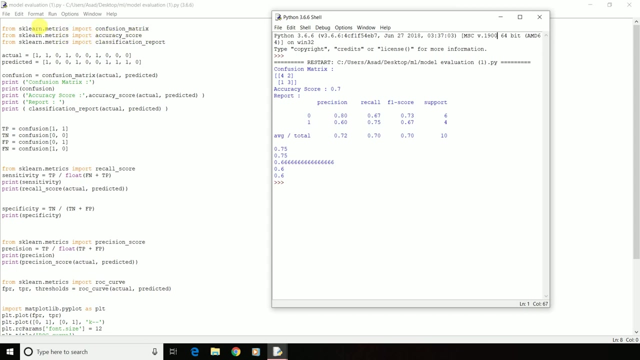 So let us try to make a confusion matrix out of it. What is a confusion matrix? We will know. So we have imported this confusion matrix function from sklearnmatrix and we have passed our actual and predicted data. To compute the confusion matrix, you first need to have a set of predictions and also the actual target values. 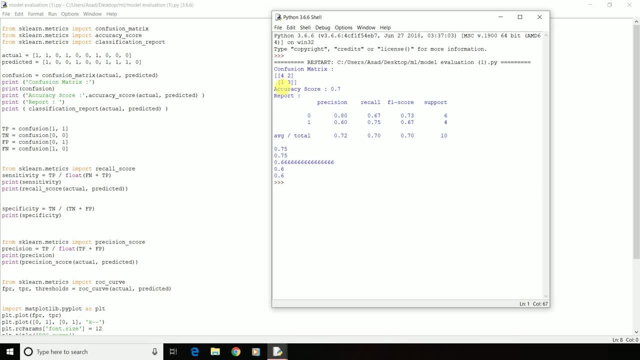 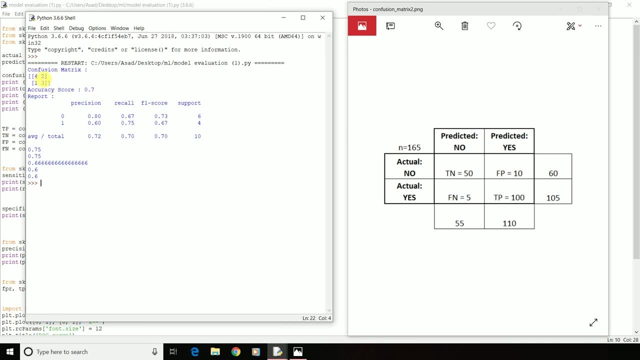 This is the confusion matrix we have got. The confusion matrix is a set of predictions. The confusion matrix is a set of predictions. The confusion matrix is a numpy array. Here you can map this particular array with this image: 4 is nothing but TN. 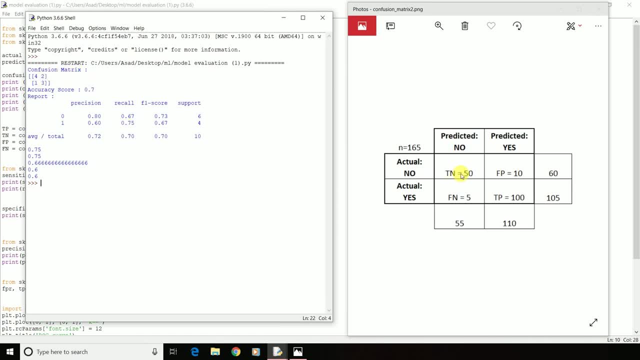 TN stands for true negative, which means your actual value was no and you also predicted as it as no. 2 resembles to your falsely positive, which means your actual value was no, but it predicted it as yes. Next 1 will be mapped to as FN- falsely negative. your actual value was yes, but it predicted 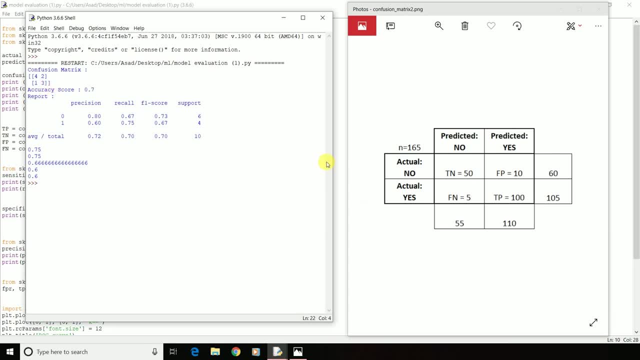 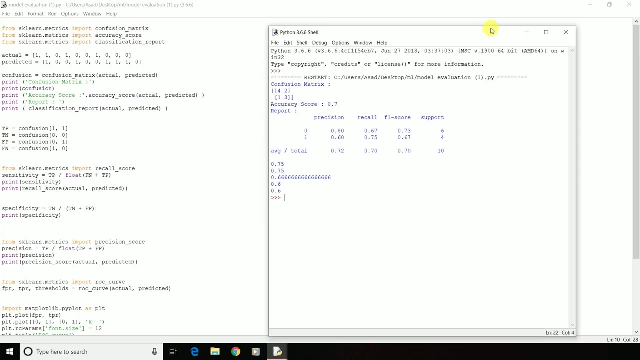 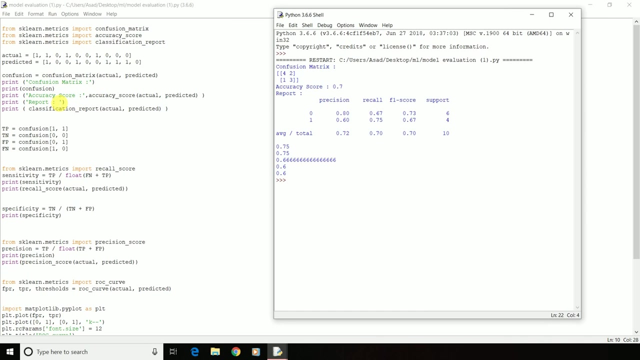 it as no. And lastly, 3 will be mapped to as TP, which is truly positive. that is, your actual value was yes, and it also correctly predicted it as yes. Now let us learn about accuracy score. It means the proportion of total number of predictions that were correct. 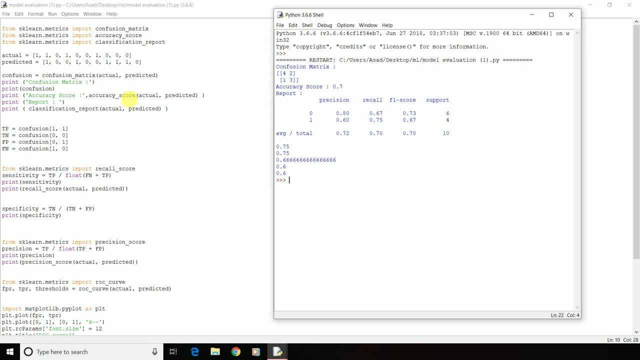 First you need to import the function accuracy underscore score from sklearnmetrics and then pass your actual values and your predicted values to it. The output will be your accuracy score. In our case, we have got 0.7 as your accuracy score. That means 70% of the predicted values were accurate. 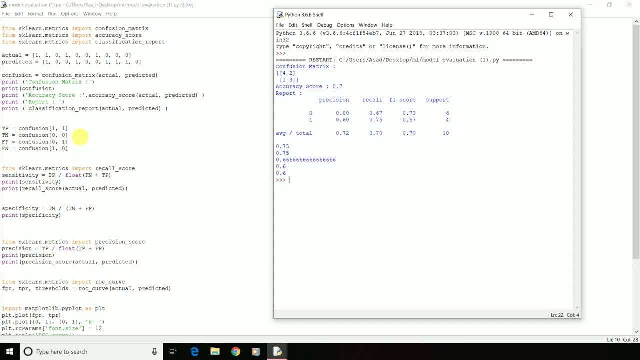 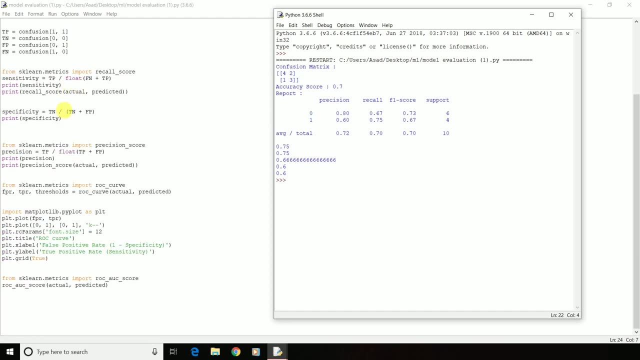 Here I have extracted the individual array values into individual variables. We have two more attributes associated in model evaluation. One is sensitivity, The other is specificity. Sensitivity, or it is also called as recall, it is the proportion of actual positive cases which are currently identified. 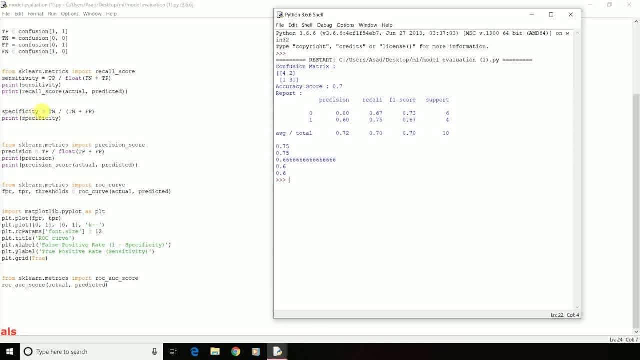 And specificity stands for the proportion of actual negative cases which are currently identified. For sensitivity, you need to import recall underscore score from sklearnmetrics and pass actual and predicted values into the function. Now let us see how it works. Whereas for specificity you need to do it manually. there is no such functions available. 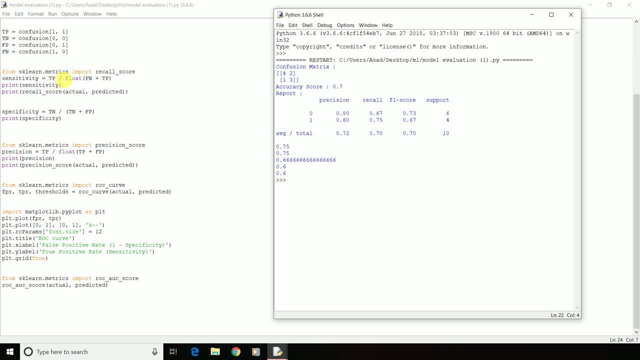 The formula for sensitivity is true- positive divided by the total row values, that is, false, negative plus true- positive, Whereas specificity is true- negative divided by the total row values- true negative plus false positive. Here I have got the output. So I have got the output. 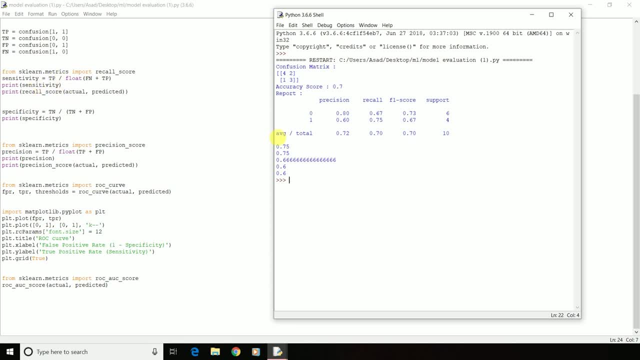 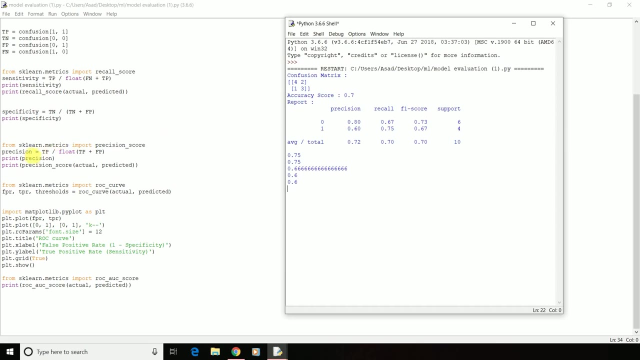 So I have got the output. So I have got the output Of sensitivity by calculating it manually as 0.75 and also using the function as 0.75. Whereas my specificity is 0.0067.. Then we have precision, which says that how accurate or precise your model is. 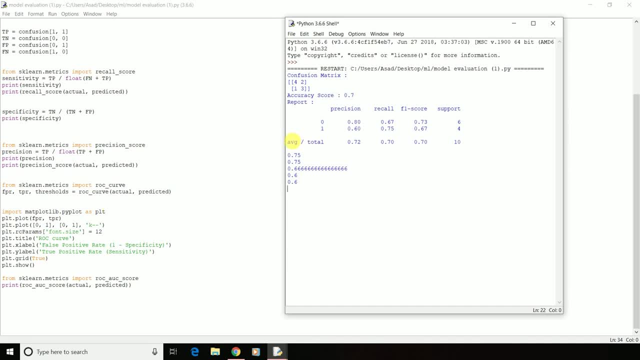 That means how many positive values were actually there among the predicted ones. So we have the following formula as truly positive divided by the total of truly positive and falsely positive. So we have calculated it manually. and also there's a function called precision underscore score, which we have. 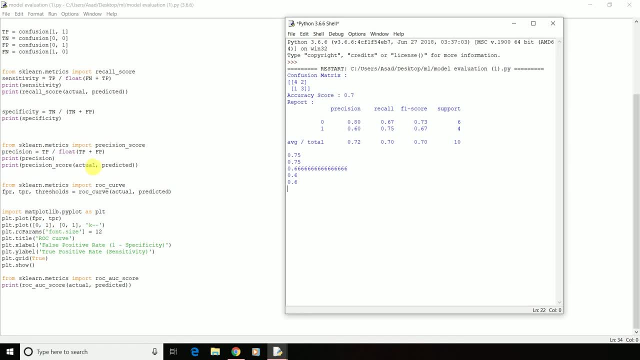 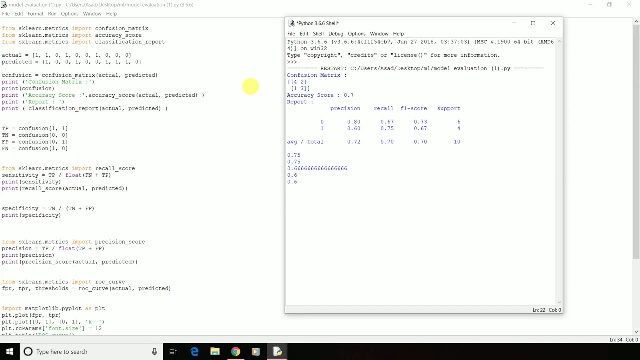 imported from sklearnmetrics and we have passed our actual and predicted values to it. So what precision we have got is 0.6- 0.6. so it's the same. We have another one function, called as classification underscore report, which will provide you with the precision, recall and other 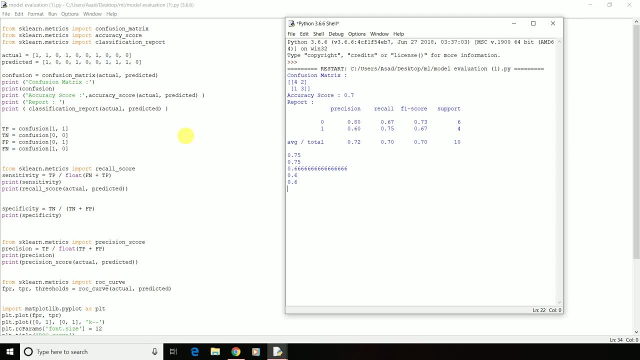 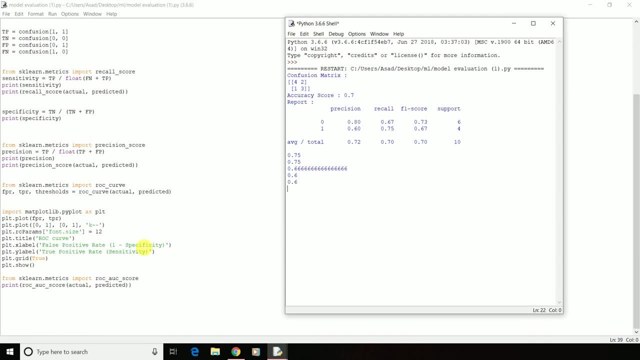 two parameters, which we won't be talking about right now, in which you need to pass on your actual data and your predicted data, and it will give you a report of all these attributes. Another method for classification evaluation is ROC, that is, receiver operating characteristic. The ROC curve plots the true positive rate against the false positive rate. The false positive rate. 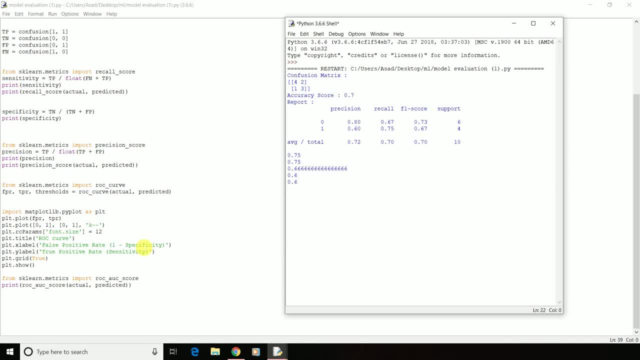 is the ratio of negative instances that are incorrectly classified as positive. It is equal to 1 minus the true positive rate. So we have a positive rate of 1 minus the true positive rate, Which is the ratio of negative instances that are correctly classified as negative. The true negative. 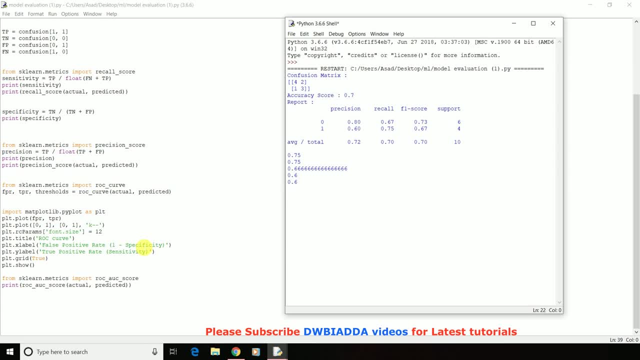 rate is also called specificity. Hence the ROC curve plots sensitivity versus 1 minus specificity. To plot the ROC curve you first need to compute the TPR and the FPR. that is the true positive rate and the false positive rate for various threshold values using the roc. 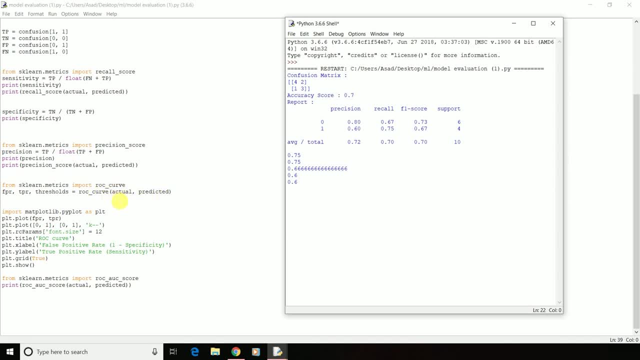 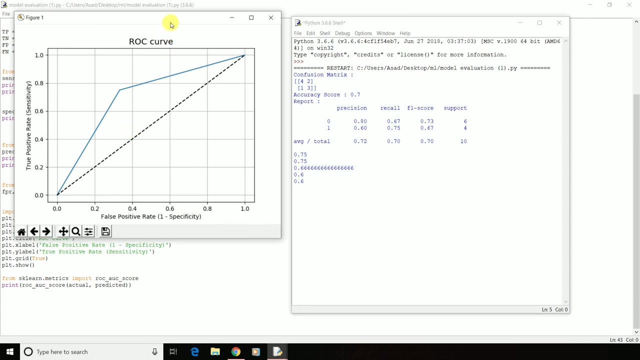 underscore curve and this function. we have imported it from sklearnmetrics and passed actual and predicted values as parameters. so this is the graph we got. the dotted line represents the roc curve of a purely random classifier. a good classifier stays as far away from the line as possible, that is, towards the top left corner. 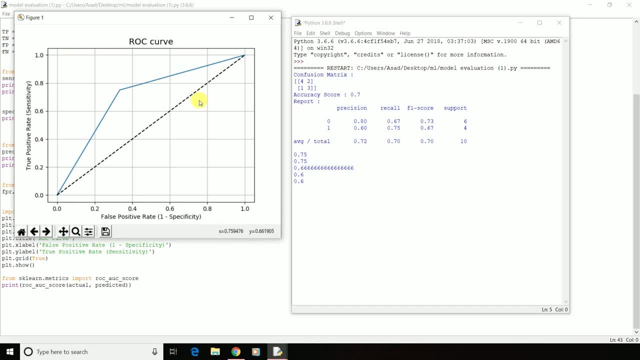 one way to compare classifiers is to measure the area under the curve. a perfect classifier will have a roc auc equal to 1, whereas a perfect classifier will have a roc auc equal to 1. purely random classifier will have a roc auc equal to 0.5. scikit-learn provides a function.